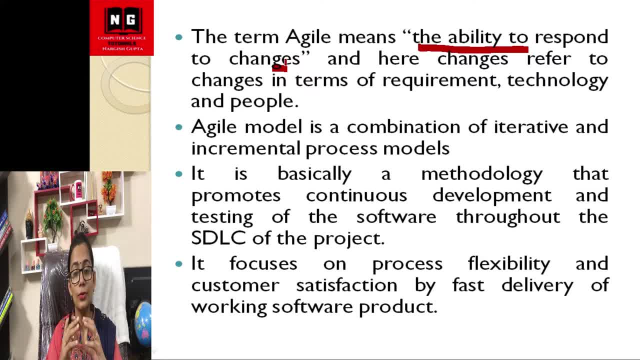 The ability to respond to changes. So what it is saying is that this is such a model which is always ready to respond to changes. The model is ready to adapt any of the changes, Either it is related to requirement, technology or the people. 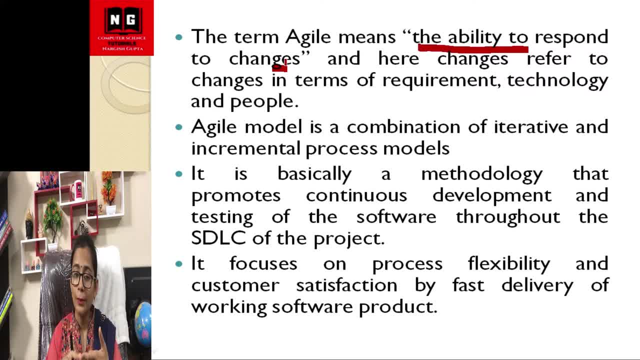 People here means the resources. If there is a change in the requirement, it also handles the agile. If there is a change in the technology, it also handles the agile. And if our resources means, suppose, if one of our team members resigns from that team, 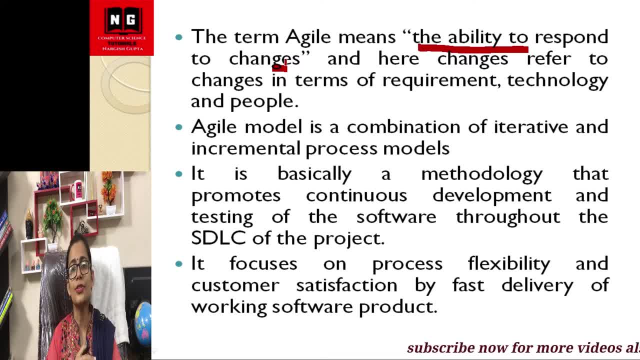 Or if a new member is added, then he is ready to handle all types of changes. This is such a model. That is why it is mostly used in the companies. Now coming to the next point, that is, the agile model is a combination of iterative and incremental process model. 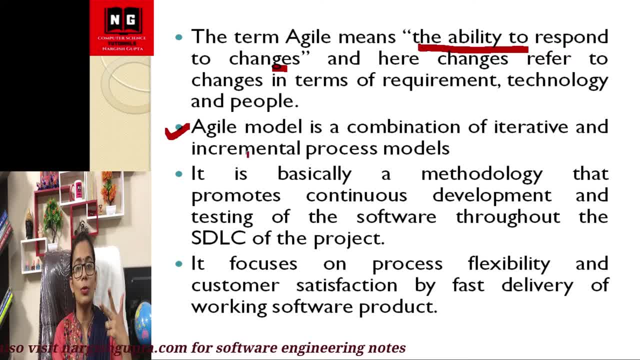 Here we have read both the models, iterative and incremental. The combination of both is the most used in it, And one point I would like to say is that agile model is such a model, which has collected the positive points of each model and kept it under. 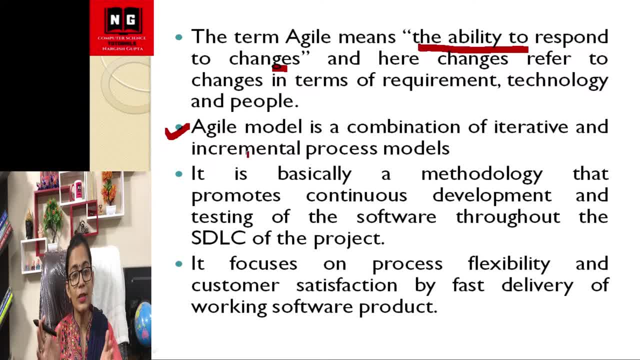 So, considering the positive points of each model, the combination of all this has become agile, And thus it is the best one. Now, coming to the next point, that is, it is basically a methodology that promotes continuous development and testing of the software. 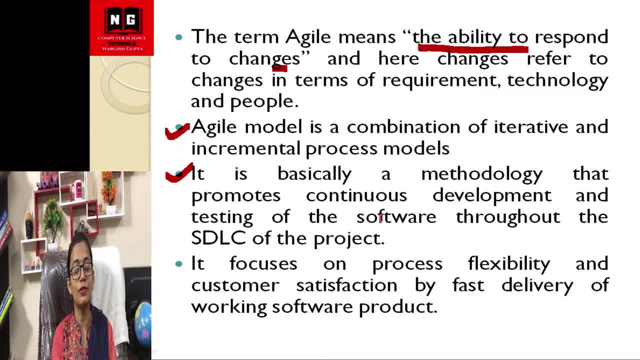 And thus it is the best one. When a project starts, its development and testing go simultaneously, And that goes on throughout the development until our product is developed. Now coming to the next point, that is, it focuses on process flexibility and customer satisfaction by fast delivery of working software. 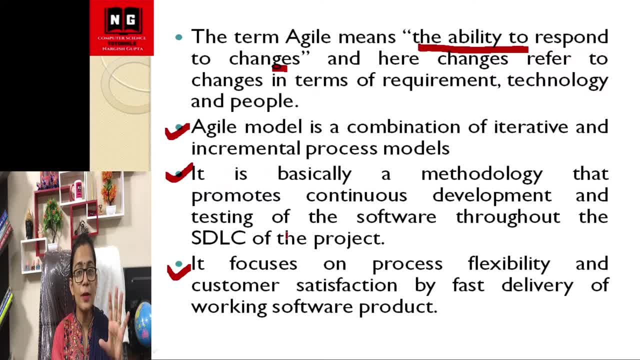 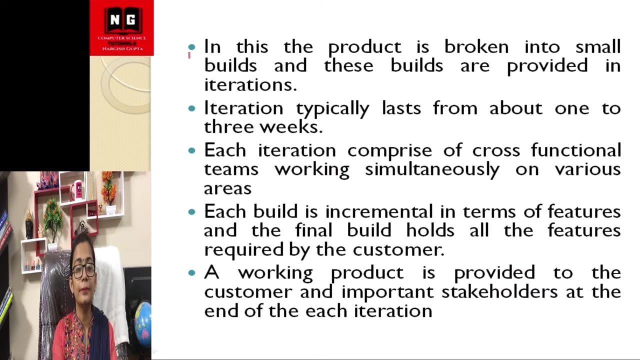 So it's technology comes first. So the main focus of this is that the process of software development should be flexible, which is the main point, and customer should always be satisfied, because customer satisfaction is the main point which the people are looking. now, Moving to the next point is that in this, the product is broken into small builds, and these 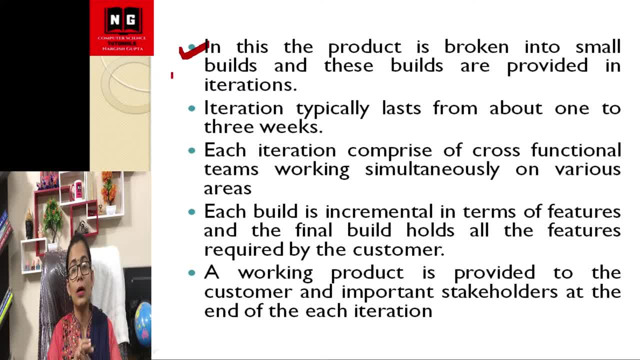 builds are provided in iteration. So how our agile work is done, that our product or our software is broken or break into different builds, like we divide our project into modules and we build them in each iteration. Iteration typically lasts from about one to three weeks. 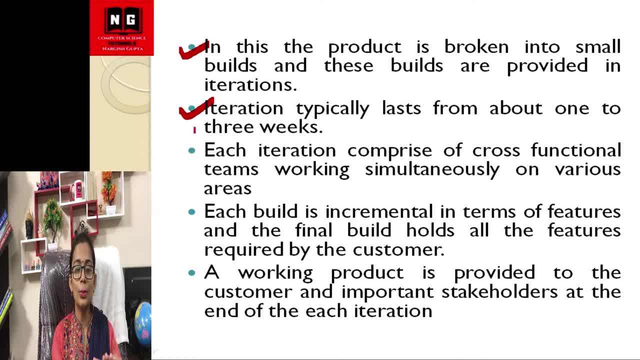 It means our iteration is basically one to three weeks. iteration is basically one to three weeks. We can say here that our iteration is two to three weeks. this point over here should be two, So our iteration should be two to three weeks. and our product is being made again and again. 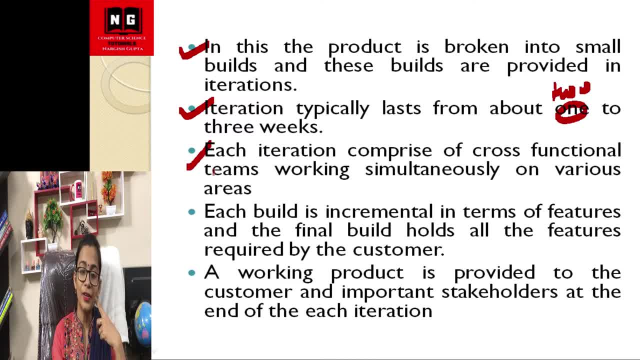 in iteration. And the next point is that each iteration compromise of cross functional teams working simultaneously on various areas. Here we have a point that what cross-functional teams? Every iteration has a cross-functional team that works individually on different area. And what is cross functional team here is in agile, not just a single team is a development. 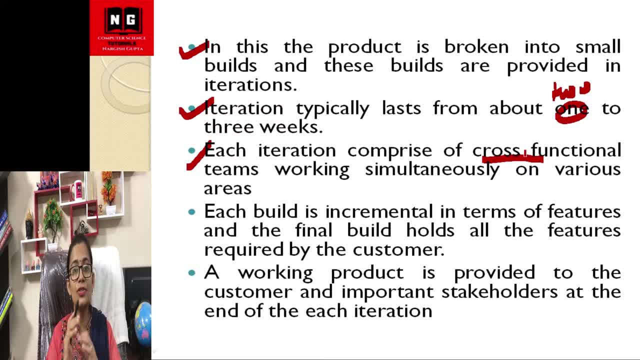 team. there is also a bifurcation of development inside the agile. For eg, For back end, For development, there is no development team. For development dependent slogan. For development, dependent slogan will be a different expertise, people will be different for ui will be different for the database and. 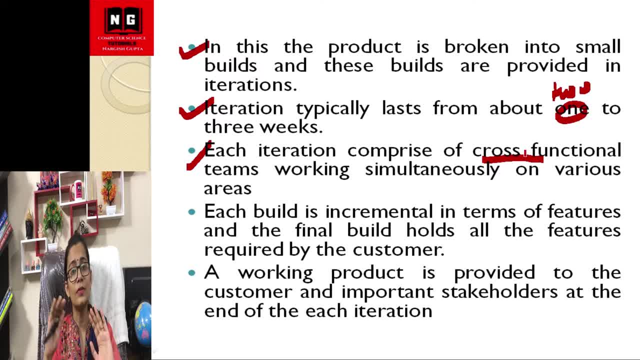 the testing team will be different. so here it comes that cross functional teams all in different things. we have taken specialized persons in our team and they are doing their own different development: UI is developing the UI, the back-end is developing the back-end and the database is working on the database. 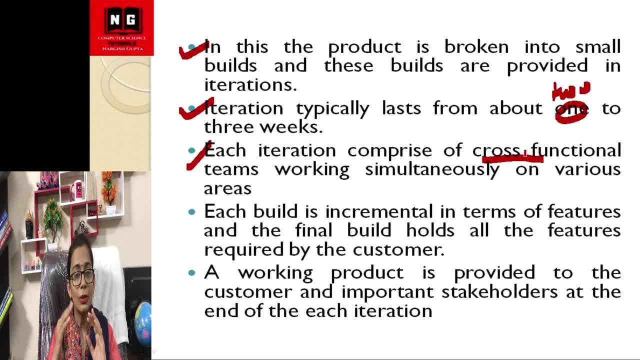 and at the end, when the product has to be delivered, of this particular iteration, combine those three things. so then they cross check with a run, so that all this is the meaning of what is basic and what is cross functional team, and this is the very important part. that is why our Agile is working very well and its output is also very good. 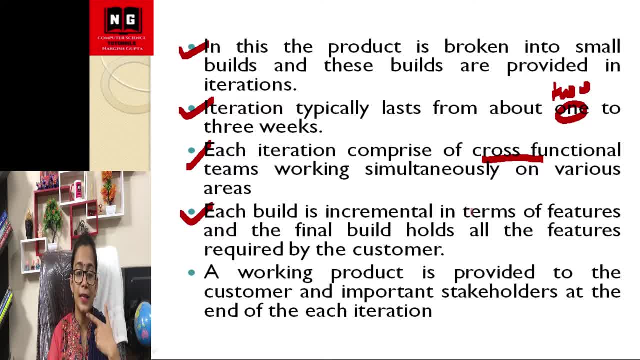 now coming to the next point is each built is incremental in terms of features and each built is a Sentence building iniance in the final built. and actually this is the way that we work out the work- work on application and the team, and I'll give institutions the feedback and implementations. 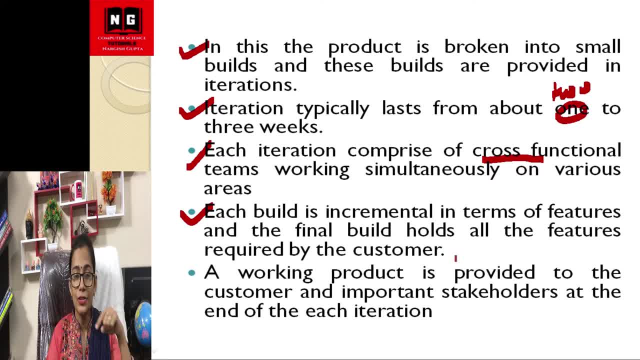 holds all the features required by the same iteration. a key same iterations, barbara use, or you took your a higher iteration. pay a bill to nickel. we hire a iteration, perfect for you. so increments may have a belt military here or your last increment over. that is self-understood. kivu full features co. 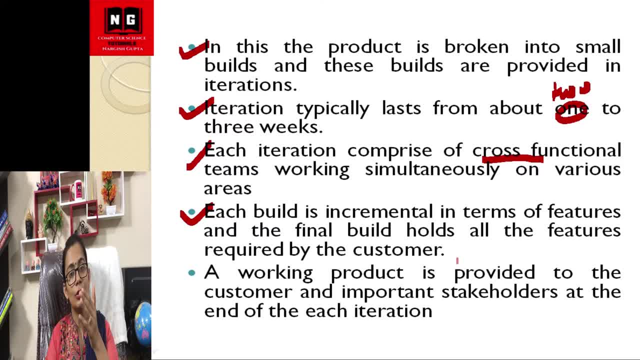 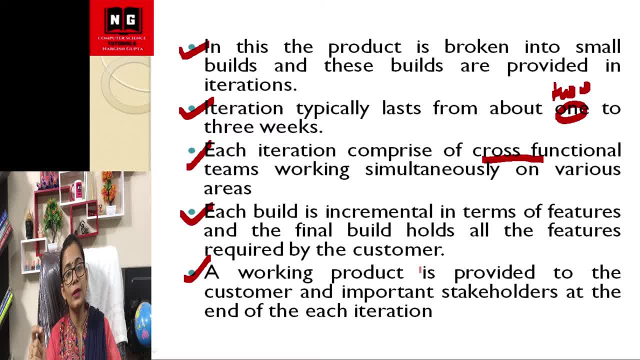 iteration. her iteration: pay a conversion of software. hum provide kardatian kiss ko apne customer ko ye main point, a key am a customer co provide kardia. her iteration to jokey. last iteration, a melega who fulfilled software meleka. a fulfilled product, meleka. but her iteration: pick a karamek. 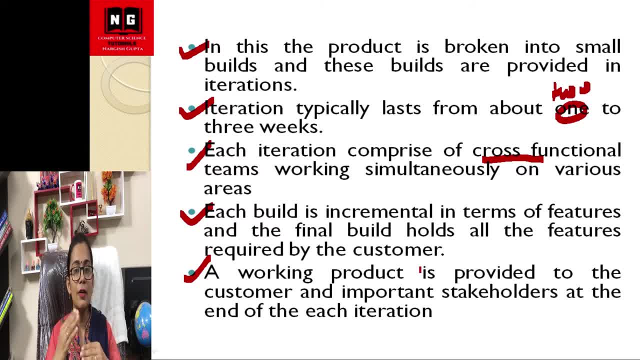 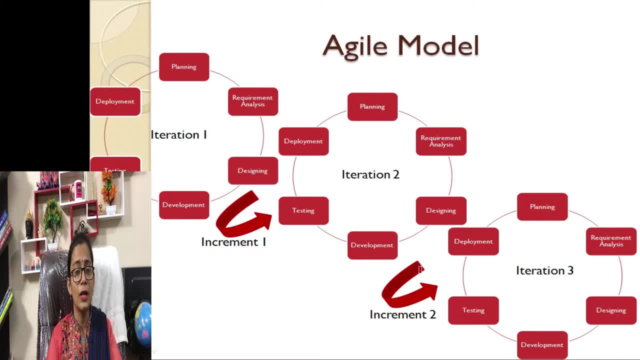 part of software, a part of product. joy deliver carter at the head, apne customer co. now coming to the agile model diagram of the hoppy is point for clear turn a kiss cheese co Joe Mara. point the iteration or increment hama. yet a incremental or 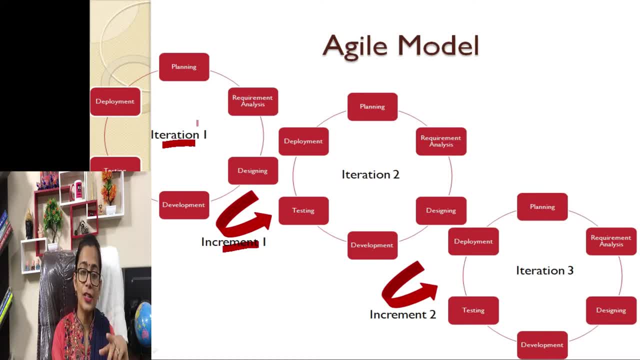 iterative model, kaiya combination iteration case away. yes, same phases. this may follow curry Jo Marie SDLC. key phases of cap planning, requirement analysis, designing, development, testing, deployment- these are the same phases, saki same planning. ma'am may start kara kia Chukka study case. a product me, kya product a? 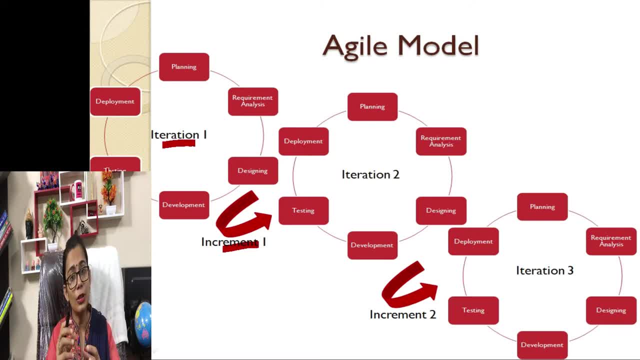 hamner division, curly ethnic division. no Nick, a bad one to this particular just part pm walkedannya vales planning k accord in Joe me or decide karo ski requirements ko gathered karo se can point packer k requirements. who gather karne ke bad? hamkei karane designing casio. Karni asky us key designing pivot. 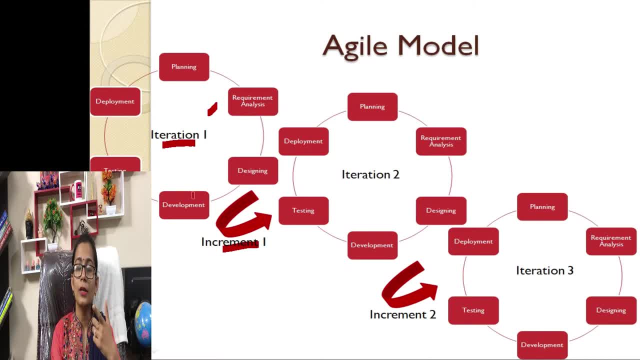 Karamon a designing case, that rikki okay for us ke bad hammeh authorising this. i mean kees teri ki of you feel it's good that I can see here for you guys, if you, When designing was decided, we did actual development of it. after development we did testing and after deployment. 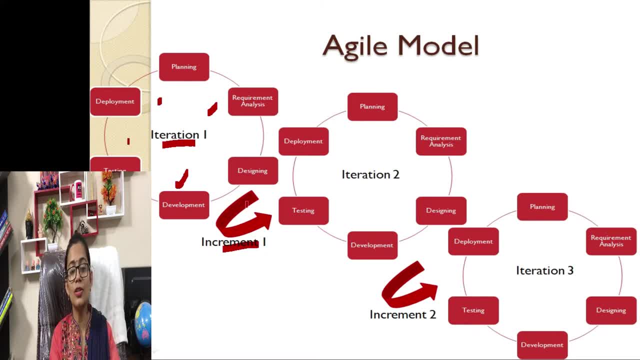 When we are going from one iteration to another iteration, an increment is coming here, So one version of our software is developed and given to the customer. So on every iteration, on every increment, we deliver a set of software or a part of software to the customer. 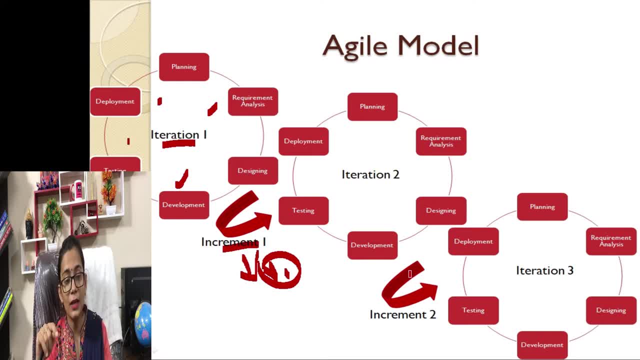 Through this meaning it is iteratively working. So in this you can see that every time there is an iteration, every time we are planning, every time we are designing, So in this we are ready to handle all types of changes. Thus this helps us in developing a better software. 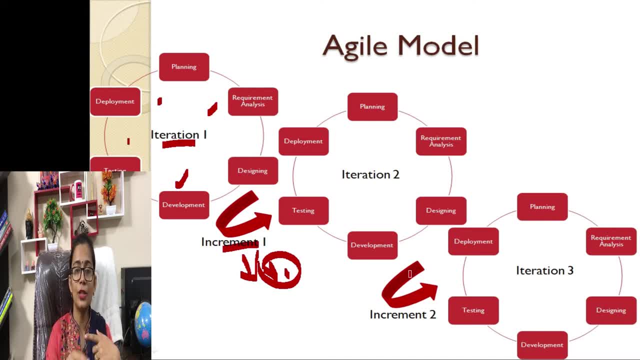 Better model. plus we are getting feedback from the customer again and again, Because we are getting feedback from the customer on every iteration. So the involvement of the customer plus the involvement of the management, plus the involvement of the team is all together So it is working properly in this way. 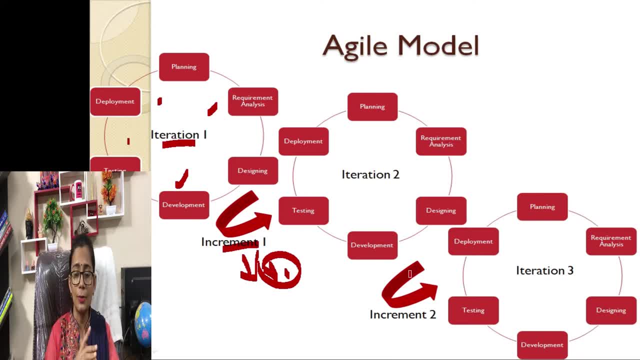 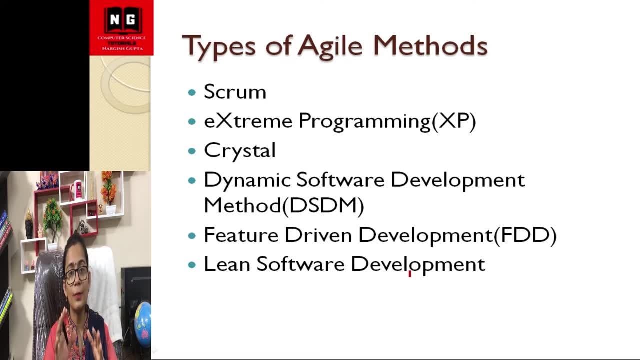 That is what the agile model is Now coming to. the next point is types of agile methods. So agile is a model of the software SDLC. It is also defining a process. So agile has defined a process which is a combination of iterative and incremental. But to follow that in agile there are many types of methods which are coming inside the agile. 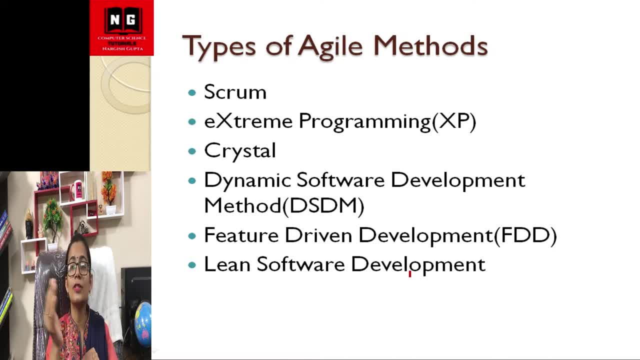 You can say that there is an umbrella, There are many things inside the umbrella or there are many people standing. So what is agile? It is an umbrella means a process Inside which there are participants. So the types of agile methods we will say here: Scrum, Extreme Programming, Crystal, DSDM, Feature-Driven Development, Lean Software Development. 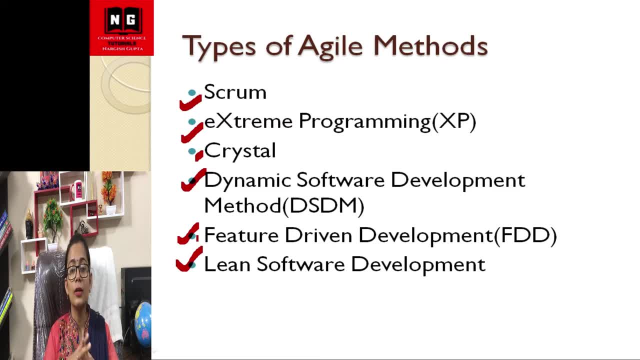 These are the different types of agile methods Which we will discuss in the next video mainly. But the main point which is used the most in this is the main point. These are the two main points Which are mainly used in the companies. So we will discuss scrum in detail in the next video. 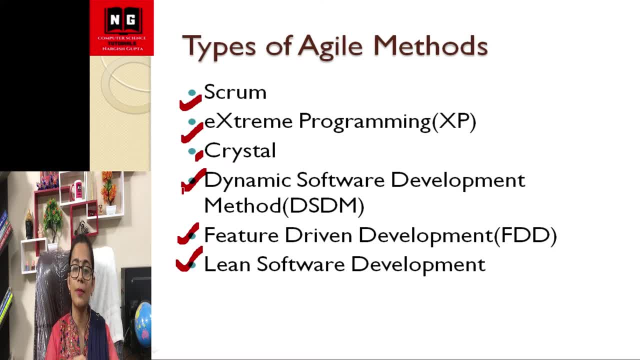 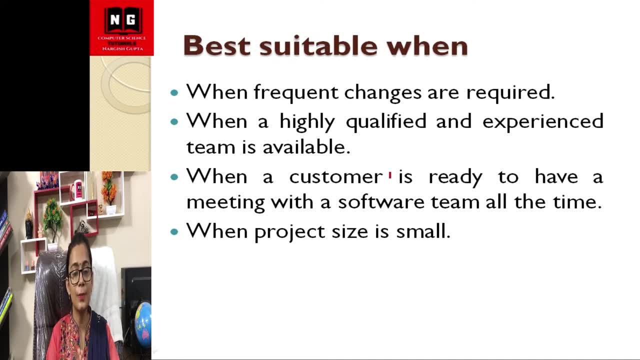 Now, here we are just looking at the names of these types, Which are the types of agile methods. Now, coming to the next point, that is best suitable when means For which type of projects agile is best. So if we see the first point in this, What he is saying is that agile is best for such projects which have frequent requirement changes. 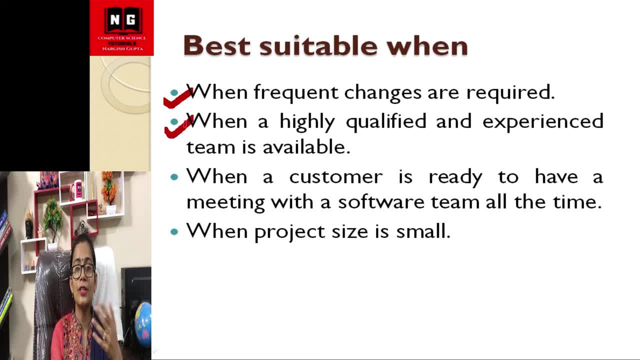 If you have highly qualified, If you have customers or team. sorry, we can say: If you have a highly qualified team, then agile is best for this. Now, when a customer is ready to have a meeting with the software team all the time, Yes, this is the main point in this. 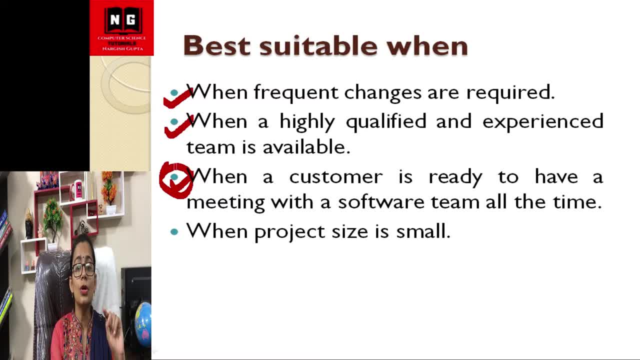 What if your customer is ready to have meeting every time? Because agile is such a method in which almost every week you are dealing with the customer, Or every 2-3 days you are dealing with the customer. Because of this, the customer should be ready to be available. 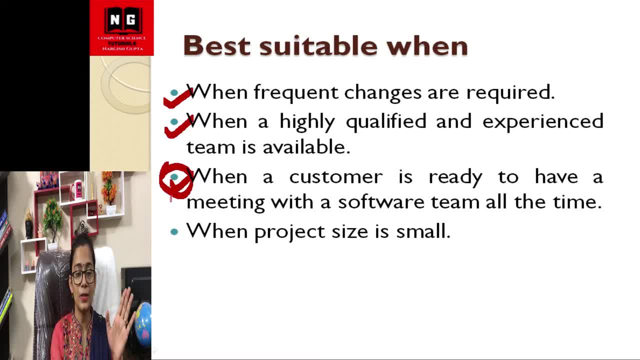 Then agile is best for you. Now, coming to the next point, that is, when project size is small. It is not like small. It is not like small, Small and large- both. It will work with both types of projects. If your project size is small or large, It will work with both types of projects. 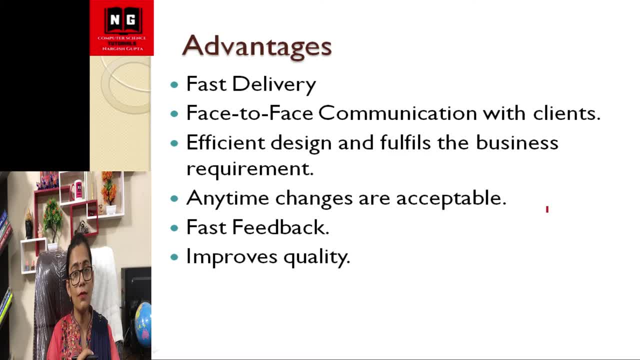 Now coming to the next point, that is, the advantages of agile. What are the advantages in this? We are getting fast delivery. Then next is face to face communication with the client. Fast delivery: We are able to communicate face to face with the client Because we are taking feedback again and again. 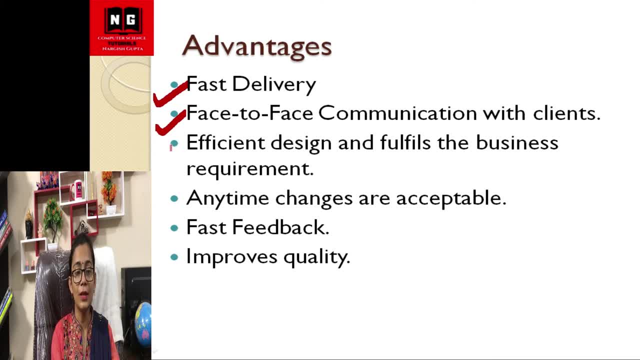 We are showing them, giving demo, and they are also replying to us Now. next point is efficient design and fulfill the business requirements Efficiently. design Why? Because if any changes come as per the first iteration or second iteration, We are ready to take all types of changes. 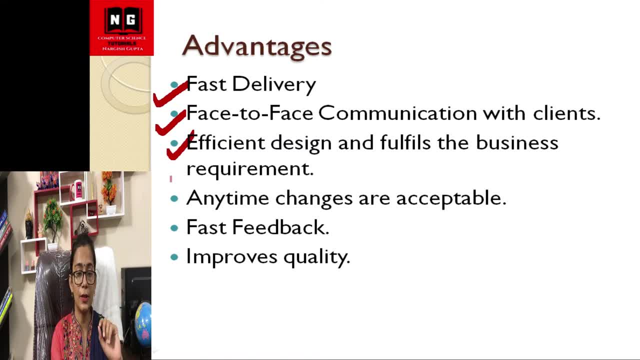 So the efficiency of the design will be good in this. Then the next point is: anytime changes are acceptable. The best point is: changes are acceptable of anything Now. next is fast feedback. Feedback we get fast improves quality. Customer satisfaction is the main point over here, And for changes we always have to take the level. 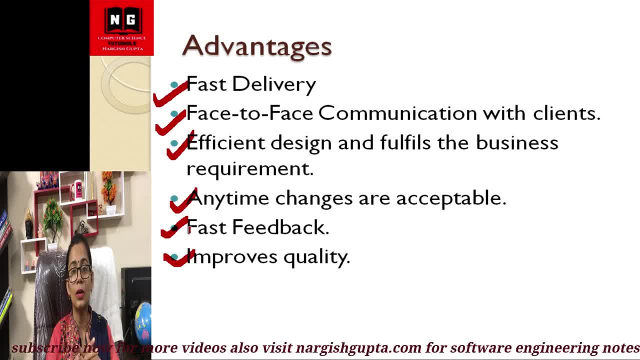 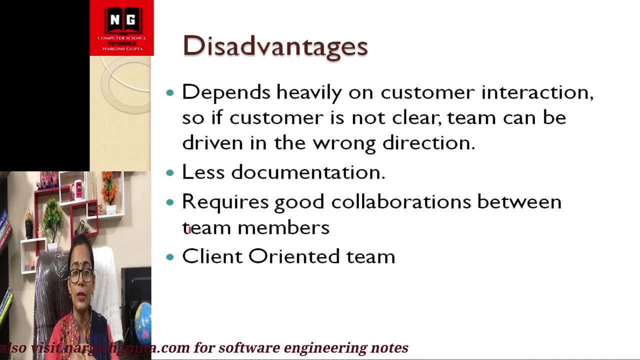 So these two points that we are addressing, Our quality improves automatically. Now, coming to the last point is That is, the disadvantages of agile model. There are some disadvantages in all of them, So this is also dealing with some. That is depends heavily on customer interaction. So if it is, if customer is not clear, 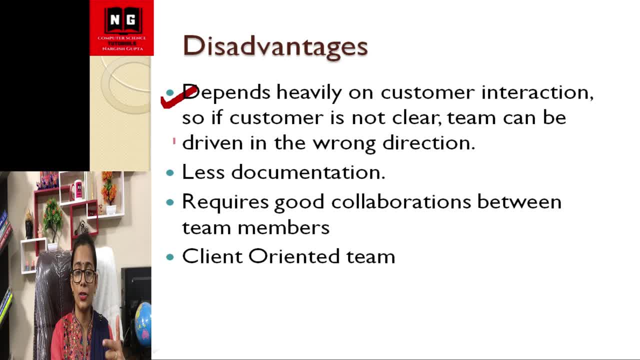 Team can be driven in a wrong direction Means we have put full trust on the customer. So if the customer is not clear for the requirements Or not clear for the project, Then there can be an issue. Now coming to the next point, That is, less documentation. There is very less documentation in this. 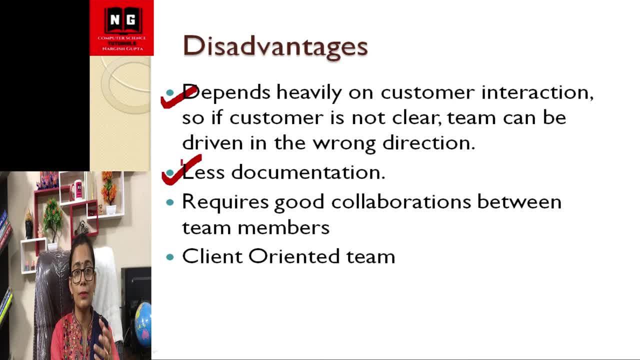 Due to which we get some issues If changes come in the resources. So there is less documentation in this, Because its documentation is completely In the end. So if there are any changes in the middle, In particular iteration, Then there are some issues. Now coming to the next point is: 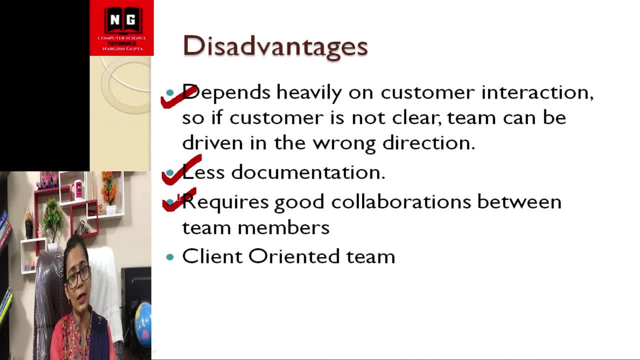 Requires good collaboration between team members. So good collaboration is required between team members, Otherwise the project gets delayed. Why? Because if the developer does not develop properly, Then how will the testers test? So team collaboration is the thing Which is required at any software project. Now the next is. 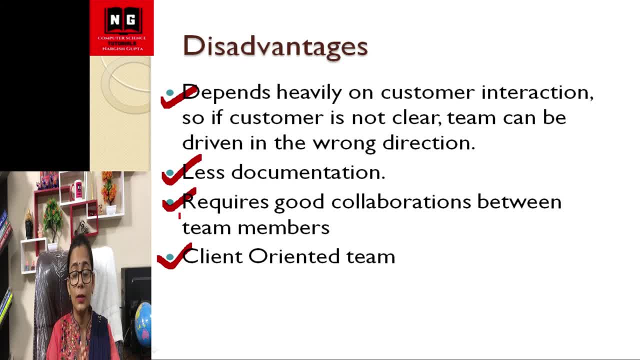 Client oriented team And the main disadvantage in this. Why client oriented team? Because we will always have to work From the point of view of the client. We can put our mind in it, But the client will not. let us put so much. Agile process is like this. 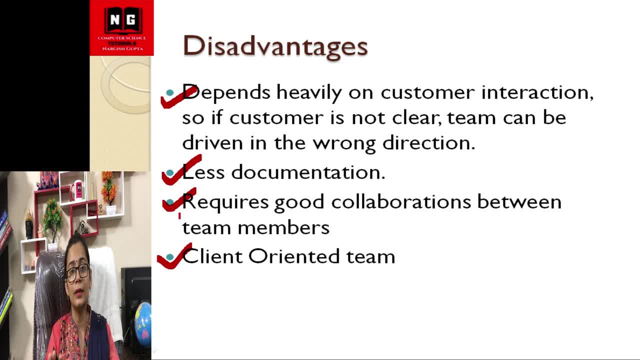 Customer has said: If this icon has to be here, Then it will be there, And after that if they say change, Then it will change again In the next iteration. But according to what they have said, We proceed first. This is the main disadvantage of Agile. So that's all with the Agile.